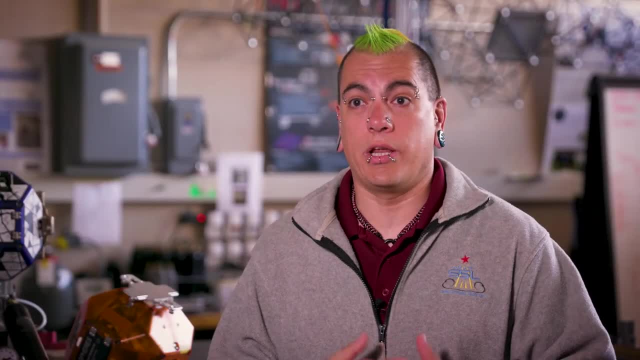 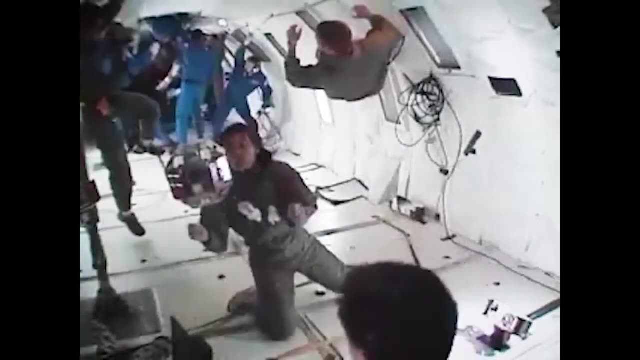 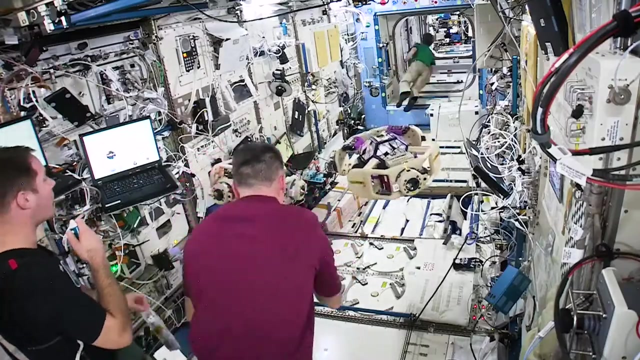 We started this concept at a time truly innovative. the first ones to ever do it: CDIO: Conceive, Design, Implement, Operate. We began that in 1999.. Since then we've done the class about ten times and at least four of them have gone to space. 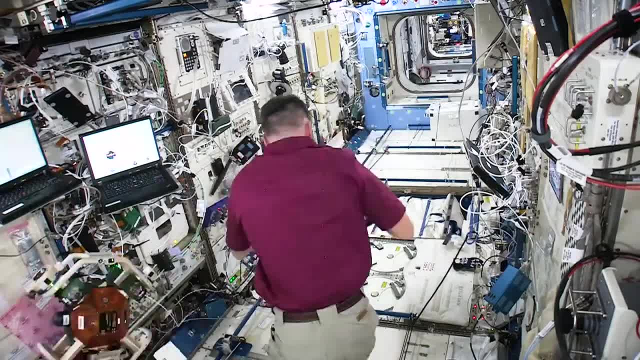 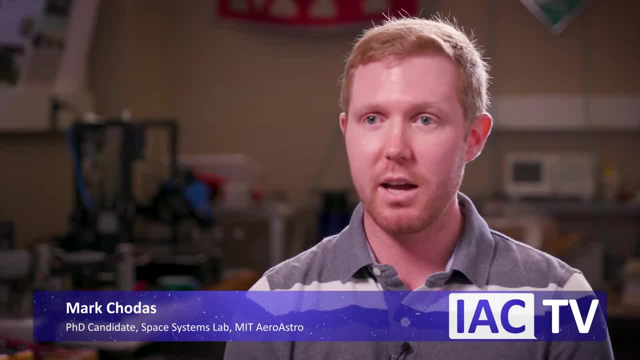 You get to experience what it's really like on a real level. It's sort of like a bit of a high-profile NASA mission. you have to meet all those requirements that the other instruments have to meet, And so that whole experience is really invaluable. 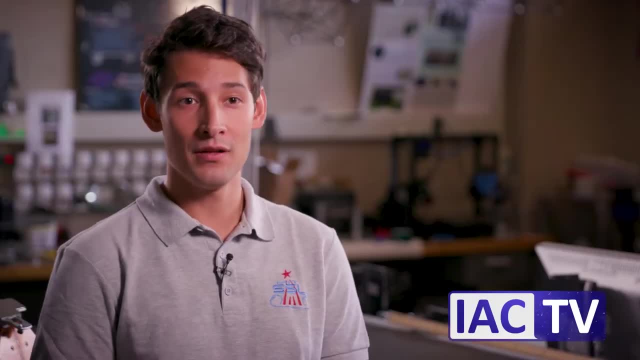 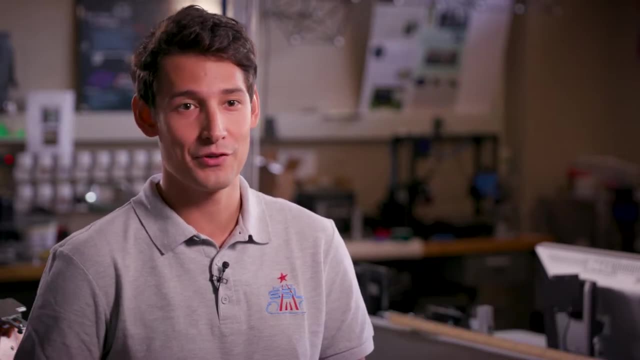 in teaching you what real aerospace engineering is like. My involvement with projects that we have here at DSSL goes all the way from the hardware level—actually crimping cables, screwing on satellite parts—all the way up to writing code for it. 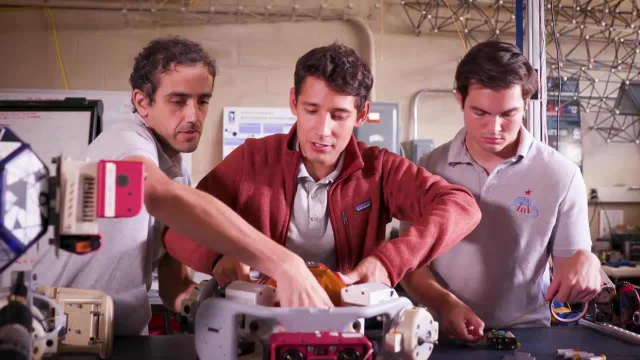 From the start, I've been working with developing algorithms so that we can test our architecture in space. We interact with the algorithm, we interact with the architect in order to tell them that we're going to be able to do it. So we've built around this new design. 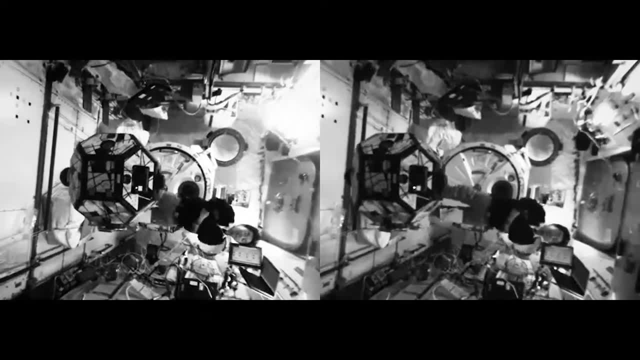 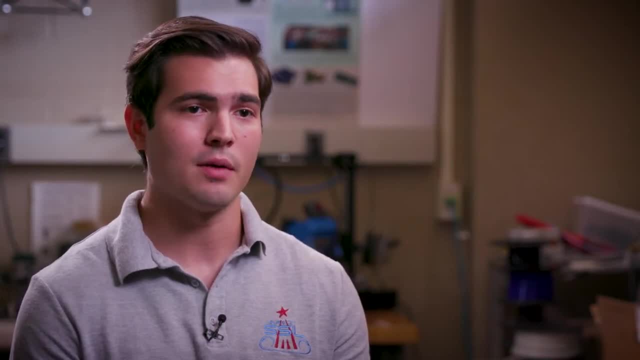 astronauts live over video feed and they unpackage our software, load it into the system and run our tests. Being able to be a part of what is the whole picture going to look like? how are we going to develop the architecture, meet requirements? I think these are really important skills that. 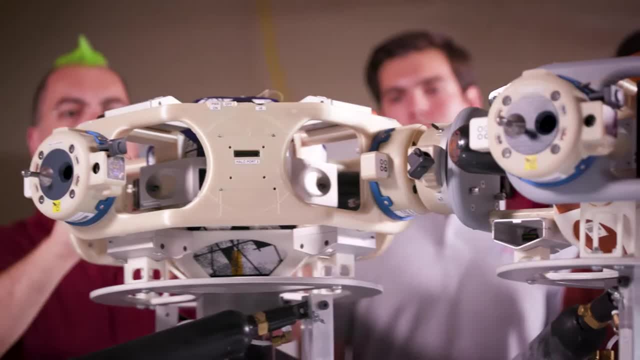 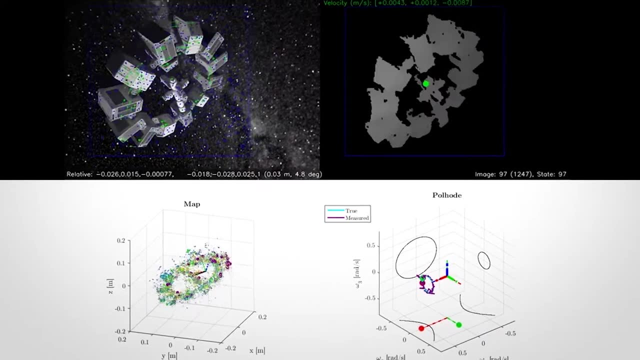 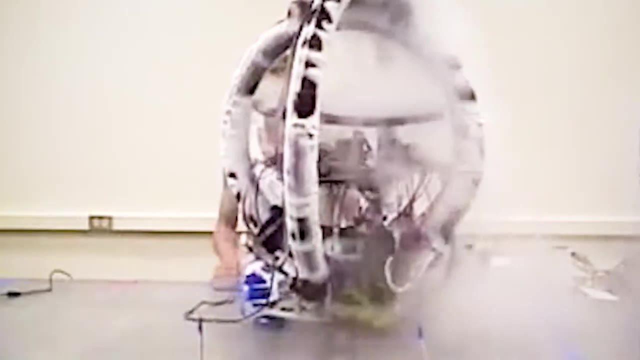 need to be developed and I think I can take into my future career. We as a lab have three main focus areas. On the one side we work with computer models of how to develop space mission. Then we do a lot of ground test beds. We build things in the ground that we test in the laboratory Proof of. 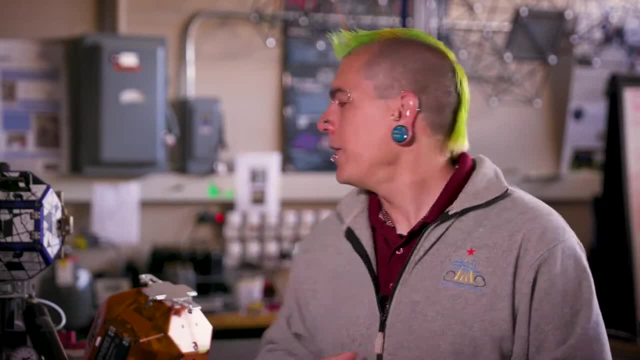 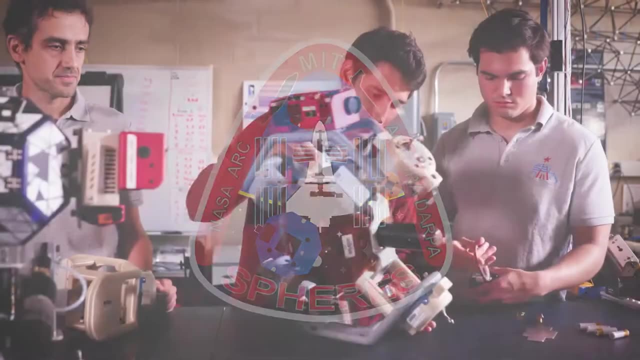 concept. can they work? The third step is things that go to space, For example, our SPHERES satellites that are aboard the International Space Station. What SPHERES is is it is a test bed. MIT decided to use the space station not to test a complete mission, but to create a testing environment to 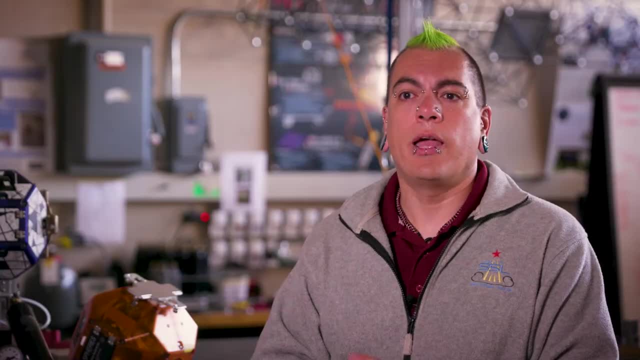 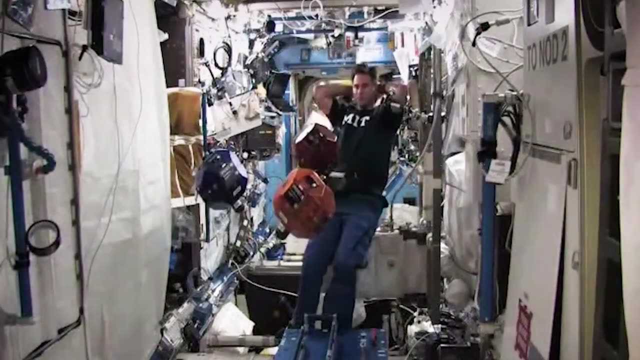 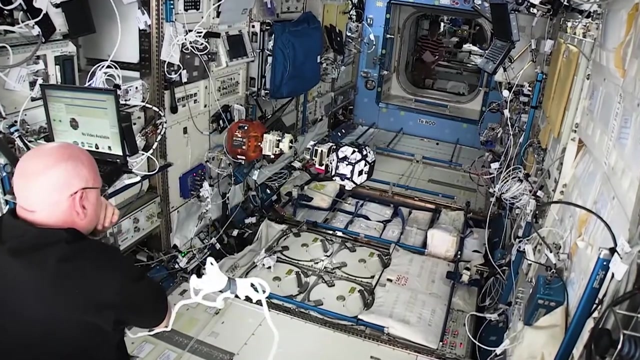 do microgravity research in space. MIT has operated over 90 test sessions doing research that goes from what we call formation flight: having satellites move together in a coordinated fashion, making two satellites dock to each other autonomously, doing things like tether formation when there's a string between the satellites. 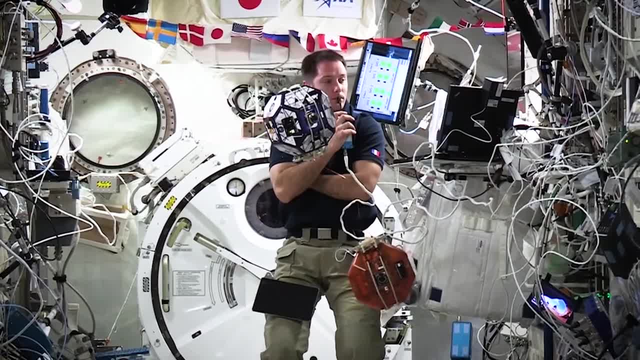 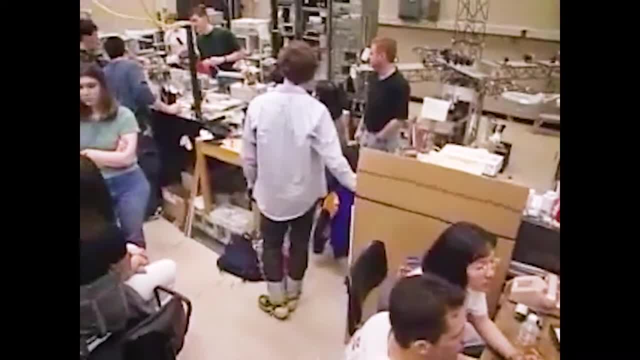 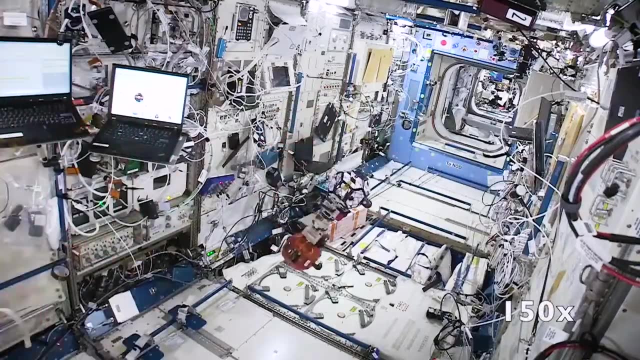 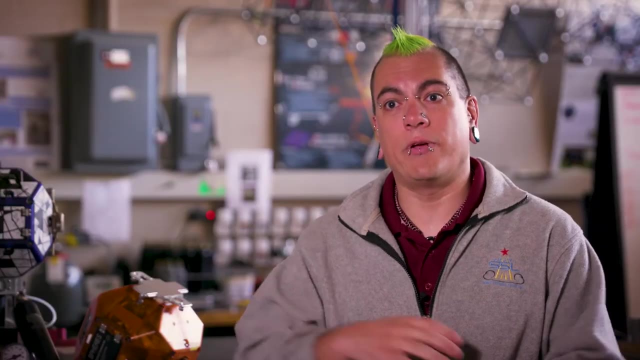 and they're flying together, keeping that tether under tension. The SPHERES program began at the MIT Space Systems Laboratory as a class in 1999.. In 2006, it got off to the space station. In 2010, NASA and the DOD made the SPHERES part of the ISS National Laboratory, making it truly a facility. 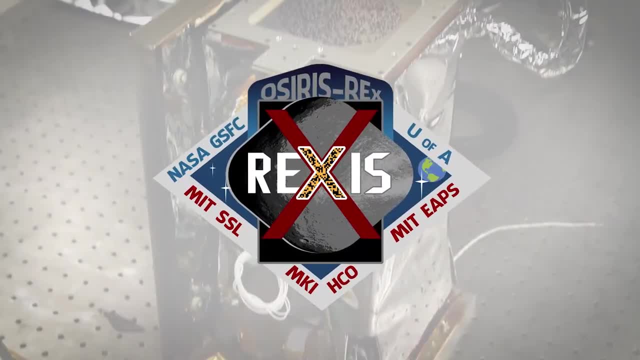 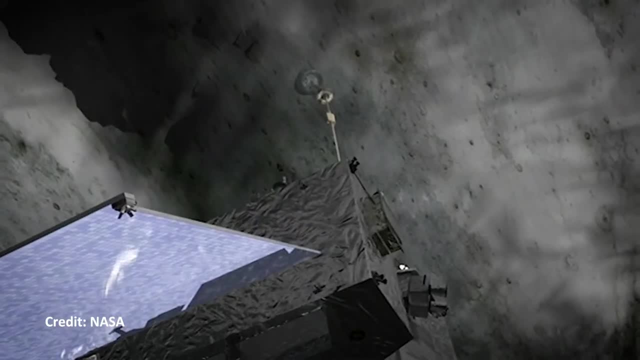 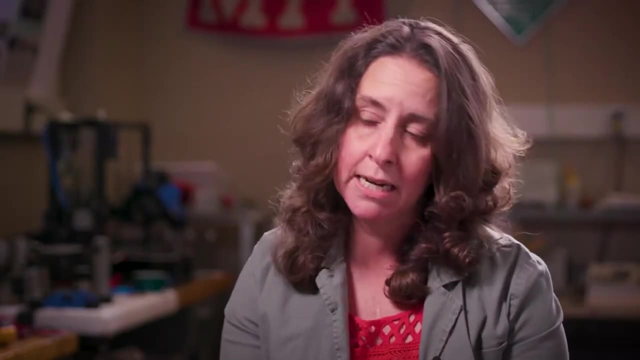 for everybody beyond MIT. REXIS is an X-ray instrument that's on the OSIRIS-REx spacecraft. The OSIRIS-REx spacecraft is going to explore this asteroid Bennu. NASA has put a little bit of money aside and said: let's see if universities can come up with a good instrument idea. and we started. 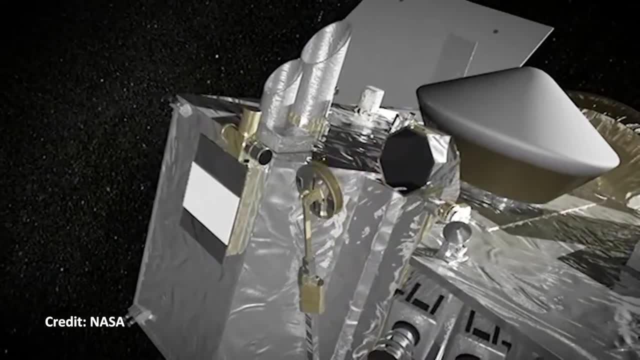 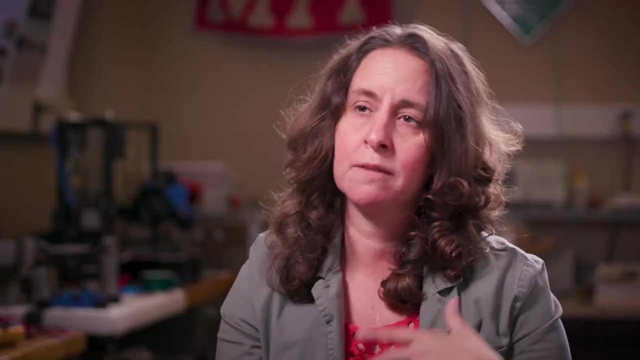 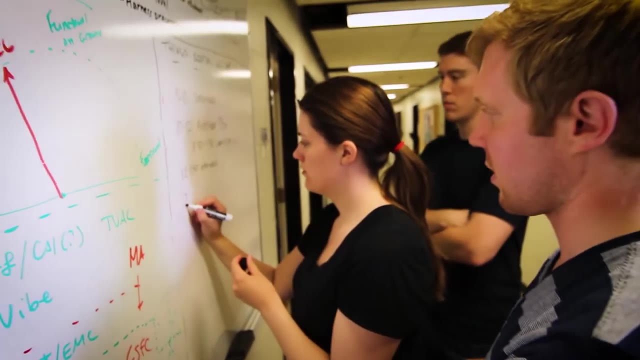 in 2012.. REXIS is going to look at the asteroid in the X-ray regime and tell us what the asteroid is made out of. So does it have iron, sulfur or magnesium in the regolith, which is the dirt that's on the outside of the asteroid? I started in REXIS when REXIS was part of the undergrad. 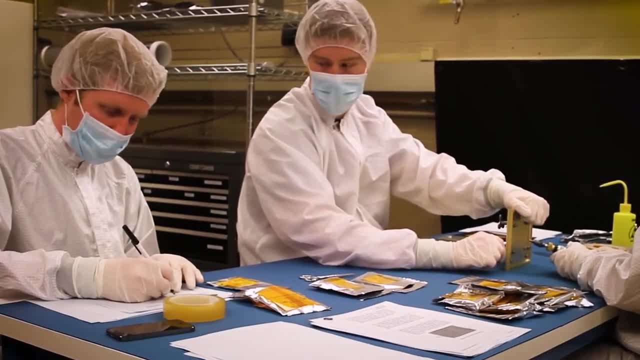 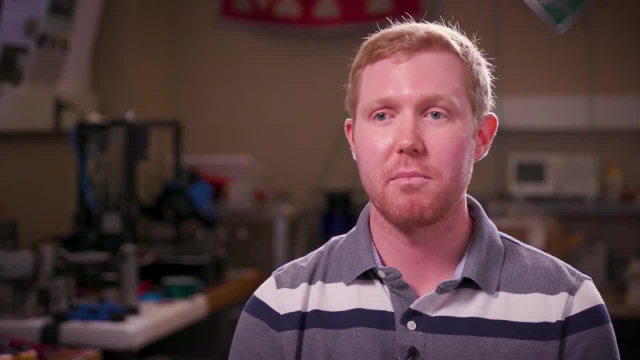 capstone class and really the experience that I got in that class was so exciting that I decided to continue on on REXIS. both my master's and now my PhD work On the REXIS project. students did everything. We designed REXIS, we designed the test program, we implemented the test program. 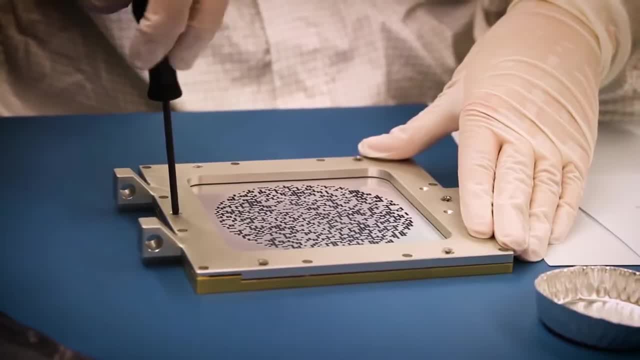 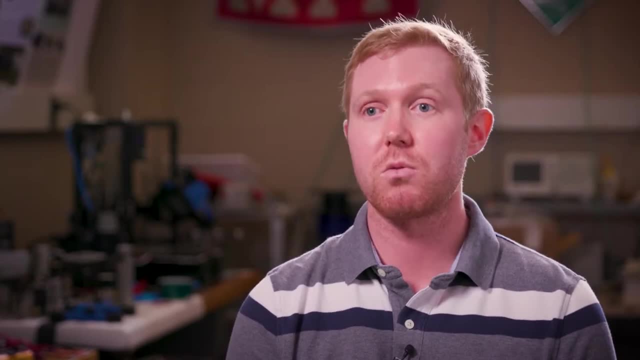 we physically built the hardware as well as contributing to the scientific analysis of our data As an X-ray spectrometer, we'll be the first instrument to get a look at the X-ray spectra that comes off the asteroid, which gives us unique insight into the elemental composition of the 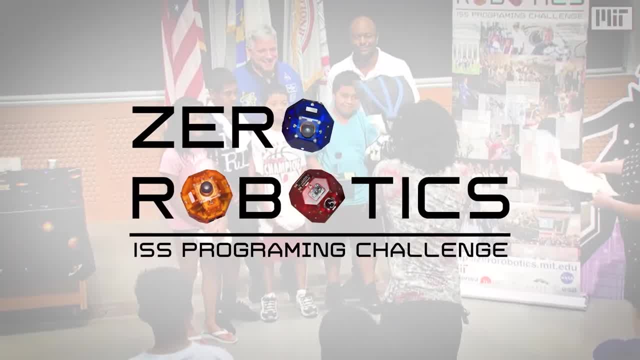 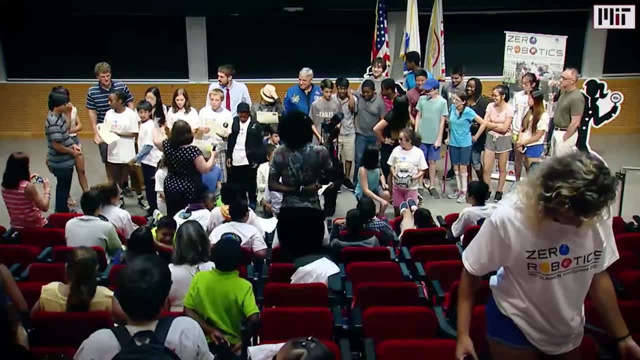 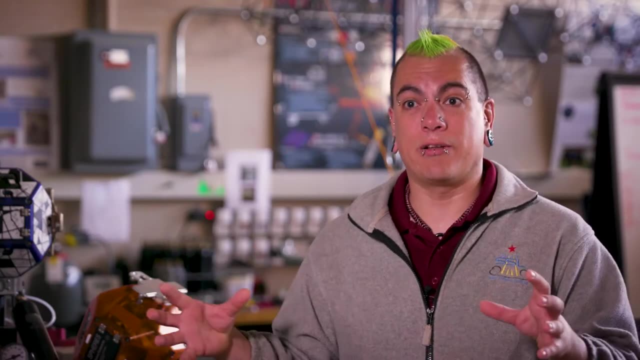 asteroid, and so we're getting data that no one's ever gotten before. The SPHERES program has educated several thousand students from all the way as young as 11 years old. We made a competition that is based on the students programming a player for an autonomous satellite. The best players in 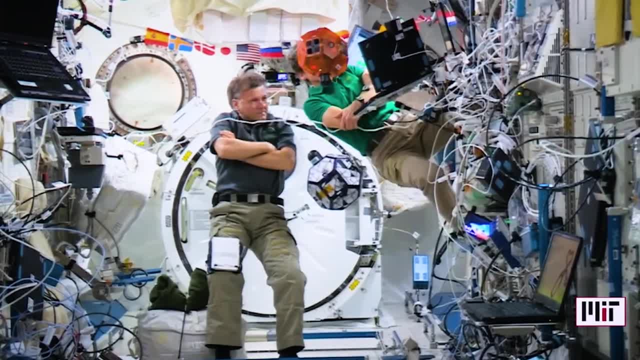 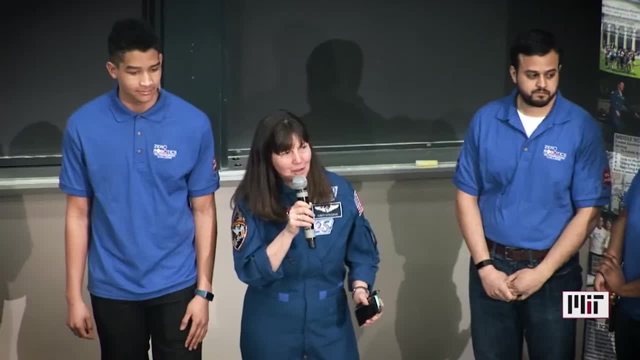 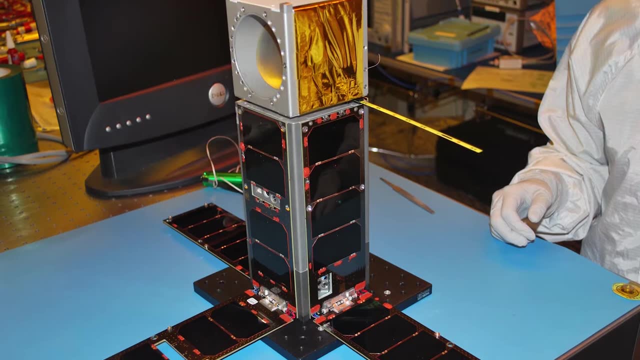 simulation, get to send their code up to the space station. Students can say: I can send things to space, I can send my software to space. Space Systems Lab and Star Lab are in a nice sweet spot. We work on missions that are small enough, where where we can hold them all in our, in our.